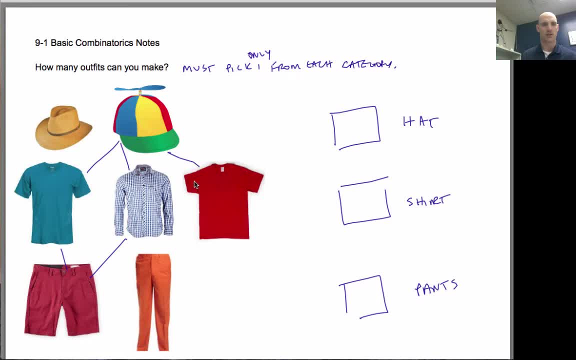 I could take this hat, put it with this shirt and this pair of pants. that's three. But then I could go through and I could say: well, this hat could go with this shirt and this pair of pants, This one and this one, this one and this one. 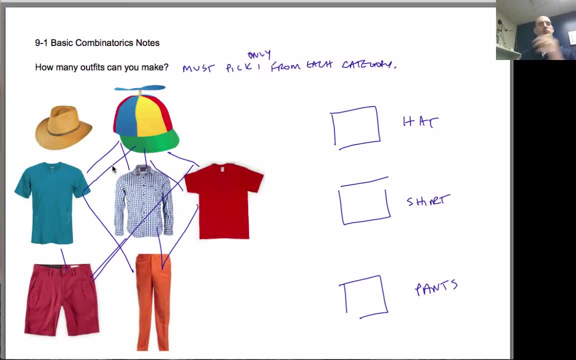 I'd have a whole lot of lines here, wouldn't I? And so there's a couple approaches that you can use to look at this, But the easiest for me is to consider how many choices Choice boxes, And you put the number of choices in each. 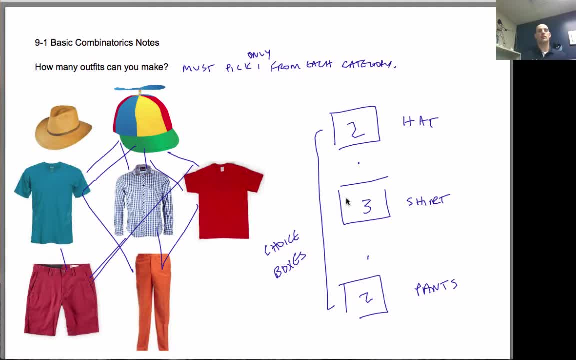 And then you multiply them. You multiply them because, let's say, you have five combinations of pants and shirts. Well then you have to multiply that by two, because that would be the number of hats you have. So any hat could go with any of the other combinations of shirts and pants. 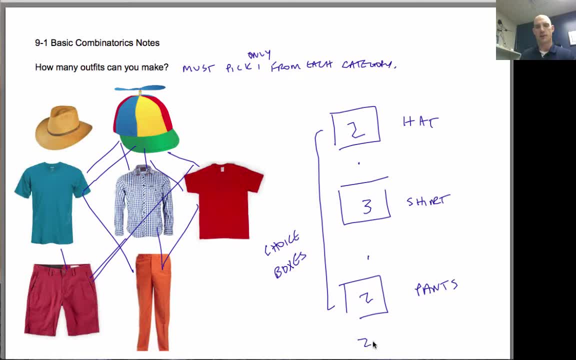 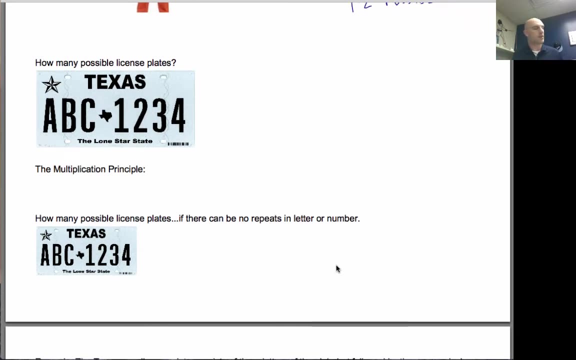 That's why we multiply. So two times three is six Times two would be 12 possible Outfits. Not asking if they go together, Just saying they're possible. Okay, How many possible license plates? A couple of considerations that we have to make here. 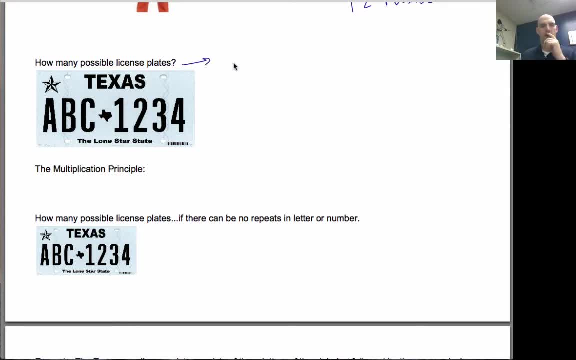 Basic example I'm going to say you can use numbers zero through nine and A through Z for any spot. Okay, So there's some license plates in some states where you have to have, like you know, three letters and then two numbers or whatever you know. so you have specific limitations. 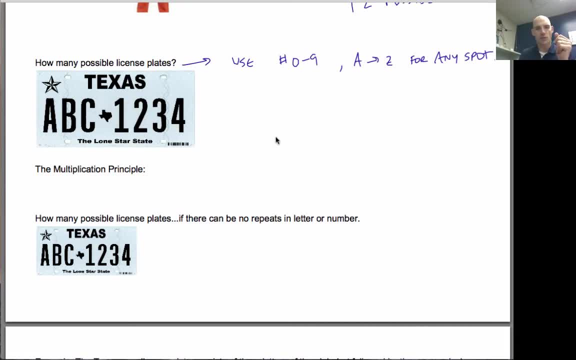 on what can go where. But if we think about it like this, we can say to ourselves: okay, I've got these slots one, two, three, four, five, six, seven, And if I, if I don't have any stipulations on repeats, meaning, oh, you can't have two. 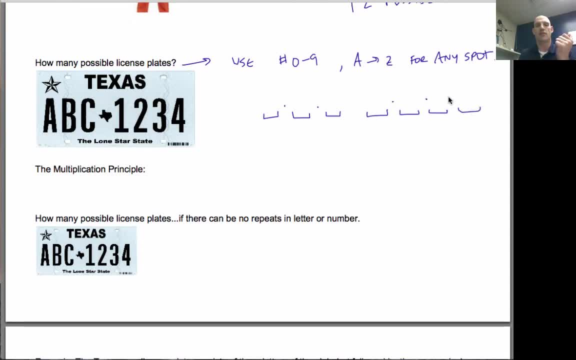 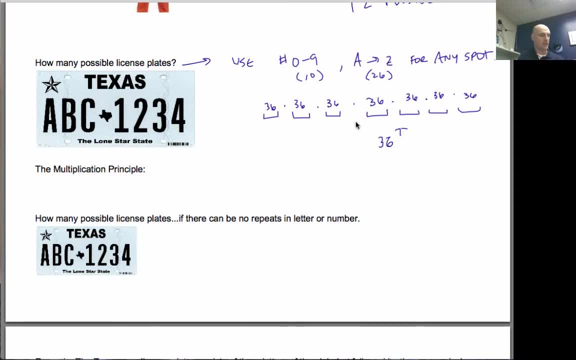 I have 36 to the seventh power And that is a humongous, humongous number. Okay, And my point is to say let me rewrite it: 36 to the seventh power. My point in saying that is a humongous number. 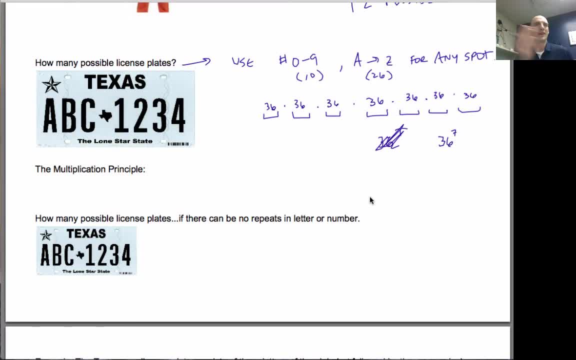 Not evaluating is there are ways that you can do this problem where you get like 200 or 300 or 400, 500 choices. We'll think about that. If you've got a license plate from the state of Texas, is my answer reasonable? 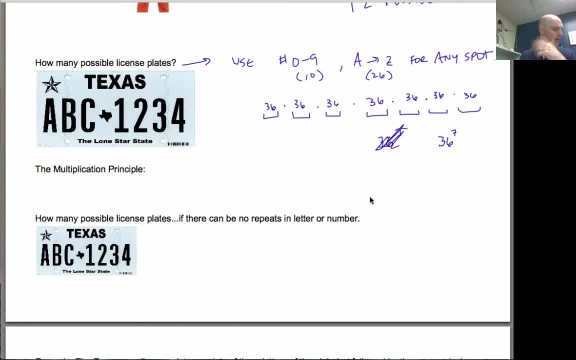 Is 36 to the seventh power reasonable? Yeah, I think so. Multiplication principle: That's basically what I've been teaching you. We're just putting a label on. I like to think about it in terms of my choices Or my options. 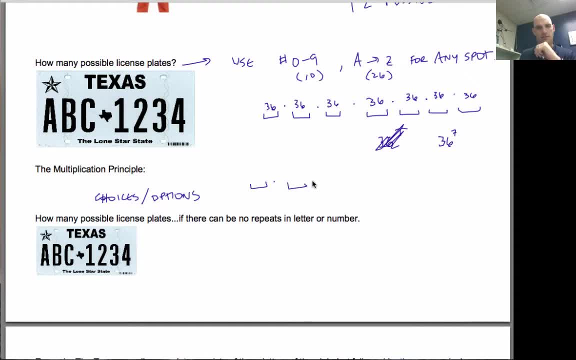 And you look at it in terms of boxes or bins or spots, And I'm going to put a dot dot dot here, because these are choices, the number of choices at each spot, Okay, Number of choices at each spot. So that can kind of help. 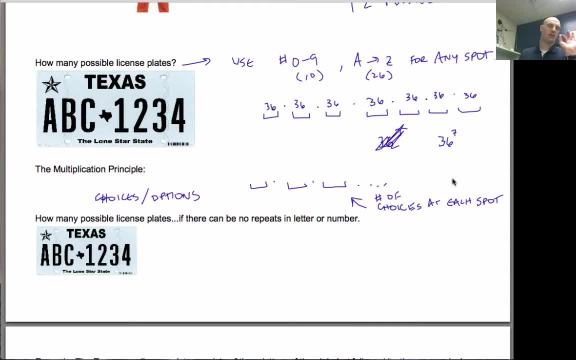 Okay, So let's think about this. Here's a variation of the problem- Pretty common variation- where we start to eliminate repeats or we start to stipulate what can be in what spot. Oh, you can't put a letter there, You can't put a number there. 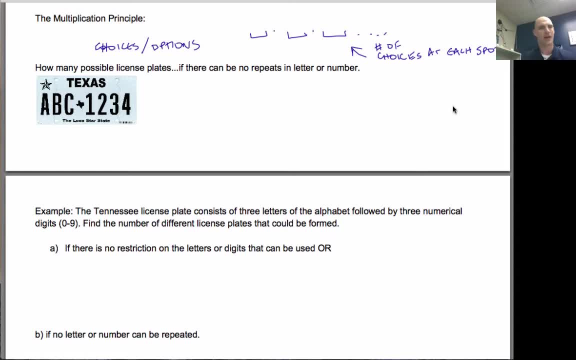 So to think about this is to really hone in on this multiplication principle. How many possible license plates, if there can be no repeats in letter or number? How many spots do I have? Well, I still have seven. It has always helped me to think about this in terms of one spot at a time. 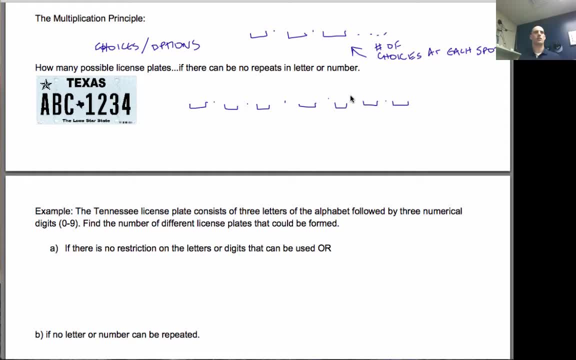 I remember in college, when I was taking a class on combinatorics, It was one of those things where I had to wrap my head around. Don't solve the whole problem. Solve it one spot at a time or one piece at a time. 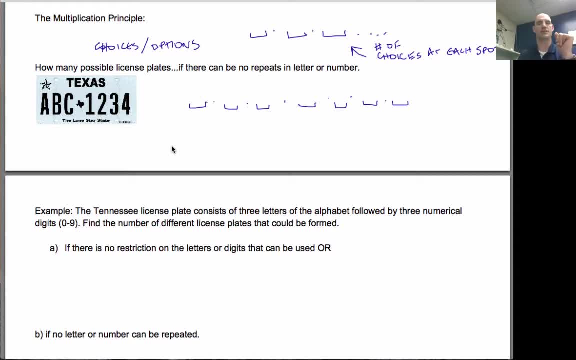 So think about it like this When I first start out: if I'm picking my license plate, how many options do I have? Well, if I've got zero through nine, it's 10.. And A through Z, that's 26.. 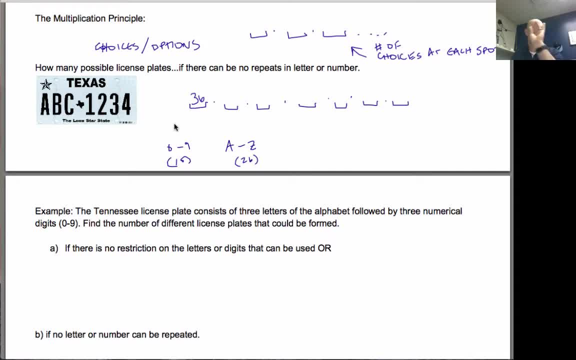 So I've got 36 options for my first letter or number. Well, when I move to my number, My next spot, if I can't have repeats, what does that mean? Well, then I'd only have 35, because no repeats. 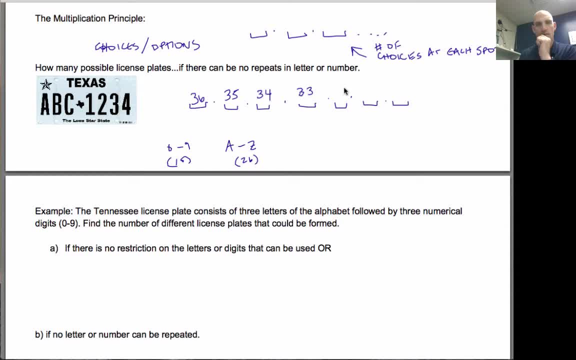 Well then I'd have 34, then 33,, then 32,, then 31, and then 30. So I'd multiply all those together. It's descending Because No repeats allowed. There's no repeats allowed, So my number of options decreases as I step down the line. 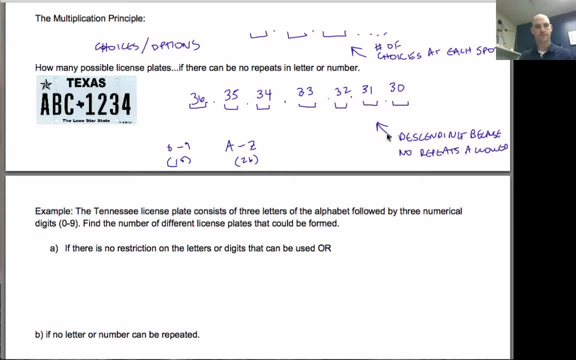 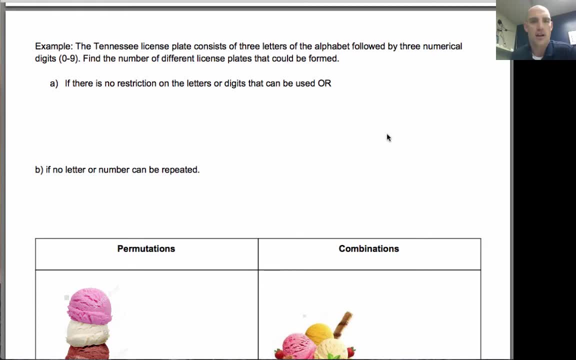 All right, Tennessee. The Tennessee license plate consists of three letters of the alphabet followed by three numerical digits, zero through nine. Find the number of different license plates that could be formed Common variation here. So If there is no restriction on the letters or the digits, that can be used, 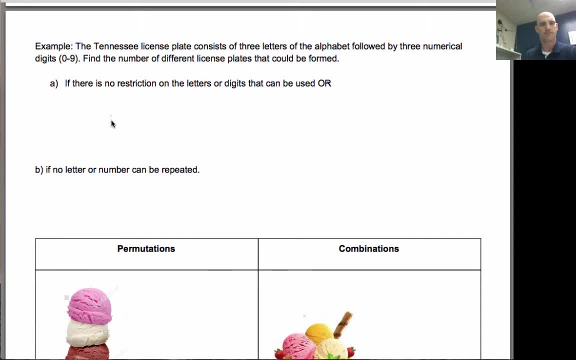 Okay, And then or goes with B. So let's think about this for a second. I've got my license plate here: Three letters of the alphabet, With no restrictions, And then four, No, three numerical digits. So check it out. Tennessee only has six characters, Whereas Texas has seven characters. Does that make a significant difference? Sure, it does. Think about my first option: Three letters of the alphabet, So that's 26.. Times 26, times 26.. Then I'm not picking letters. 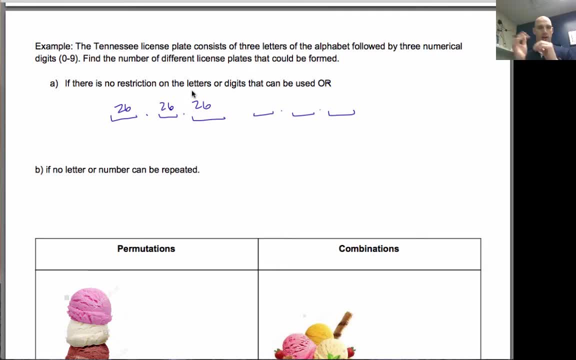 So I only have 26 because it has to be a letter. My next three must- Excuse me- Must be numbers, They must be numbers, And so you 10 times 10 times 10.. This is a case where I want to multiply this out. 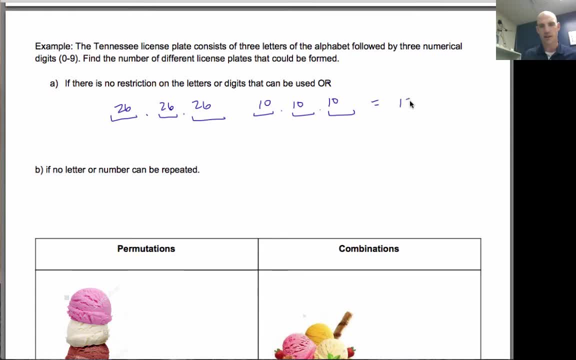 This one's very much smaller and see if it's reasonable. So this would be 17,576,000.. Obviously not taking into account personalized license plates or specialty license plates. This is just straight up Tennessee, You know 17 million license plates. 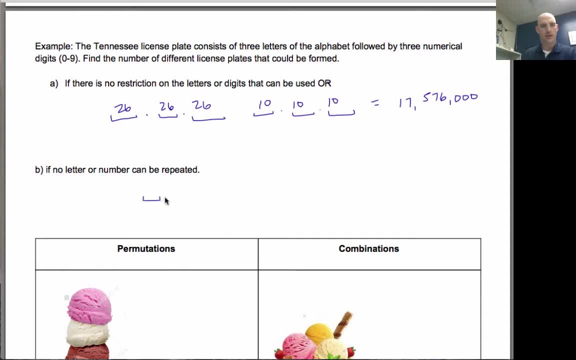 All right, Next variation: No letter or number can be repeated. This is a variation of the one above, And so I'm going to have six options, Six ways to choose again, But I'll start with my first one. I've got 26 letters. 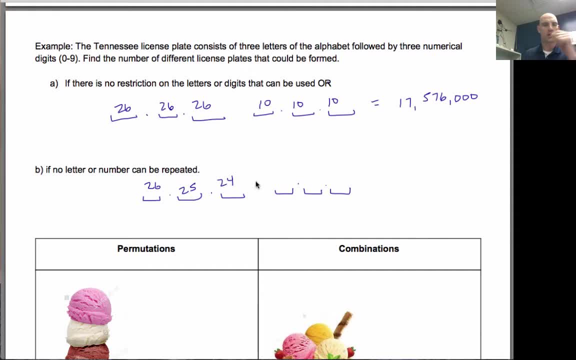 If it can't be repeated, then it'd be 25. And then 24. Then I go to 10, because I've got 10 options for my first one, But then I can't repeat that digit, So it's nine. 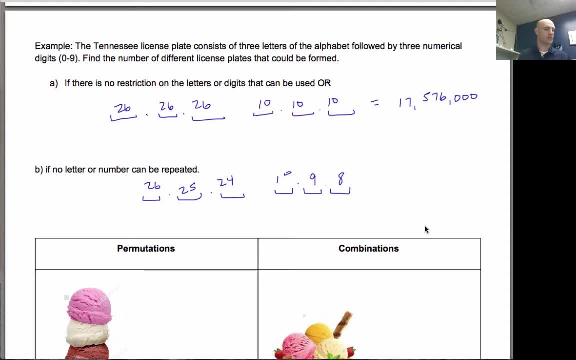 Then I can't repeat that digit or the one above it or the one below it. So it's times eight. Look at this. That small variation leaves me with six some million left, 11 million 232,000.. So just that small variation cuts out almost six and a half million license plates. that 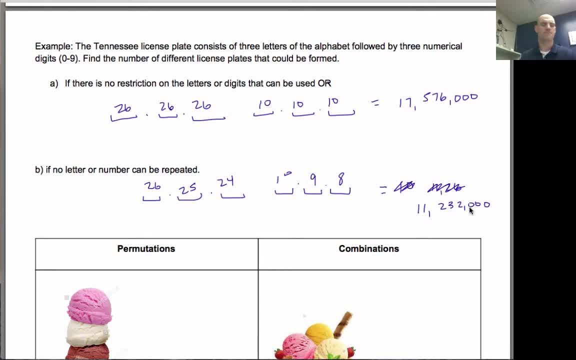 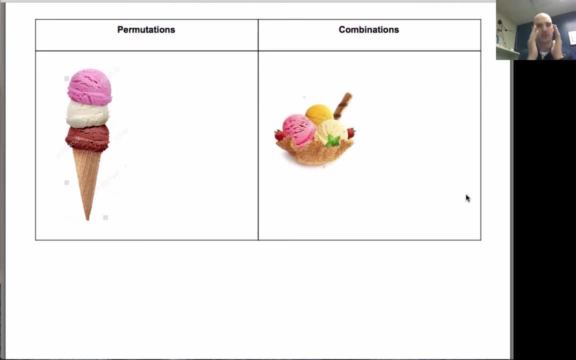 we can use. See how that's an important distinction to make. What we've been talking about is a basic counting principle, But there's different variations of this problem. For example, let me paint this picture: There's a horse race And there are 10 horses in the race. 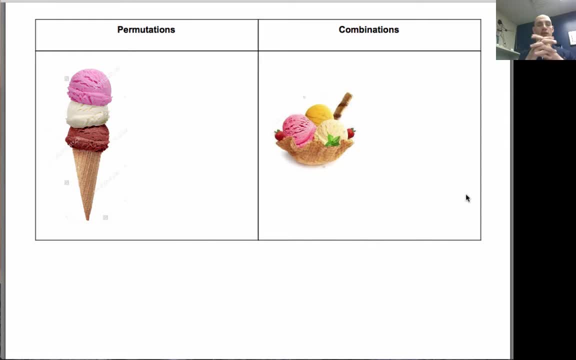 First prize, you get $5 million. Okay. So let's say they say go And the horse race is happening And you come in second place And you miss out on $5 million. Do you care? I do, Okay. 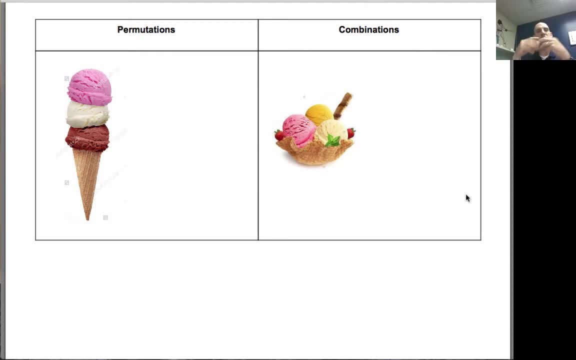 So in that case first place matters. But let's say it's a qualifying race And so you only have to make it into the top three to move on to the round where you're going to be able to race for the money. Do you care about getting first place? 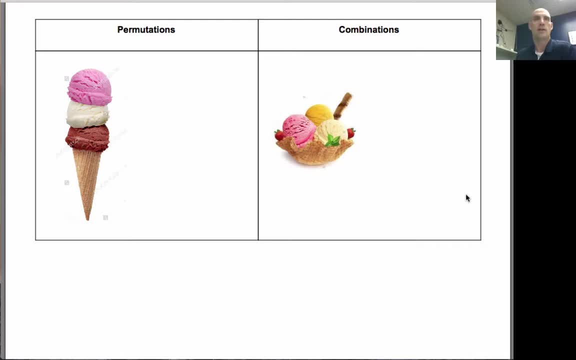 I mean, of course, maybe you want to win- I would- But really I just need to get into the top three. So whether I'm first or second or third, the order doesn't matter. However, in the championship round, the order matters. 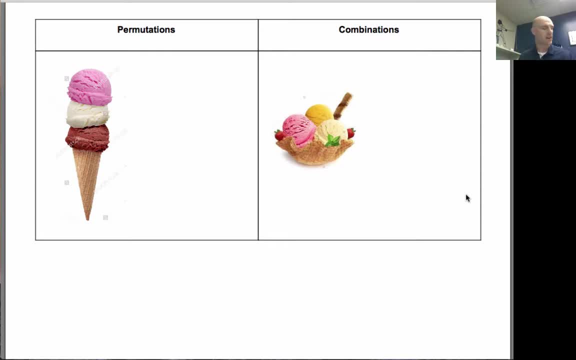 That's the difference between permutations and combinations. The best I can do is to give you a visual here. And if you think about it like an ice cream cone, As you eat an ice cream cone generally, you eat it from top to bottom right. 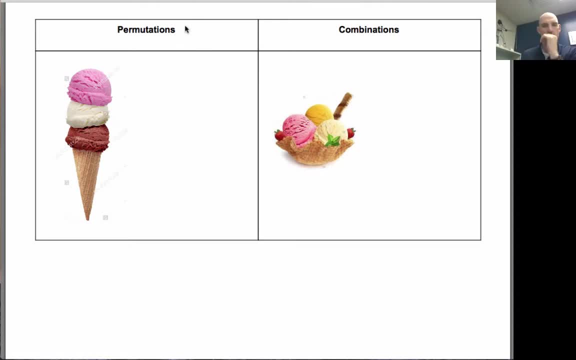 And so the arrangements. okay, This is arrangements Where ABC and CBA are different. What does that mean? That means that if I eat my strawberry first, then vanilla, then chocolate, that's different than chocolate, strawberry vanilla And maybe you don't buy into this. 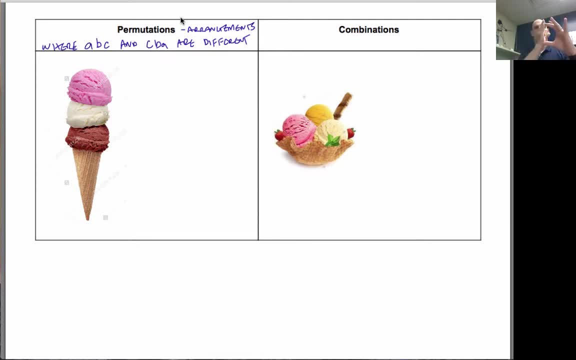 But when I was in college I used to love those ice cream sandwiches that had the Neapolitan ones: chocolate, vanilla, strawberry. I always wanted to open it chocolate side first, because I like chocolate the least, So I would want to eat the chocolate side first, all the way down to the strawberry. 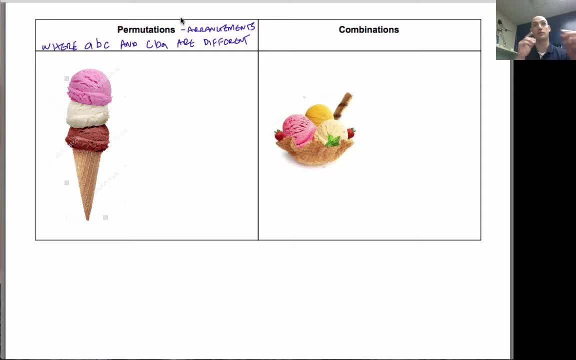 And I was a little bit disappointed, honestly, if I opened up the strawberry side first and I would close it up and turn it over. Those are different, different ways that this could be arranged. Some examples of this would be like races, where place matters. 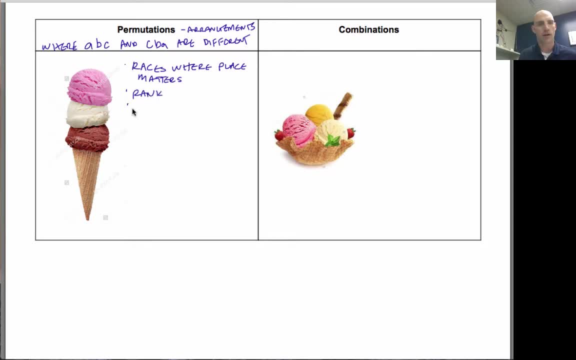 rank medals right. So like in the Olympics: gold, silver, bronze- okay. Combinations are arrangements where place matters. Rank Medals: Gold, Silver Bronze. Gold, Silver Bronze. Gold- Silver Bronze. 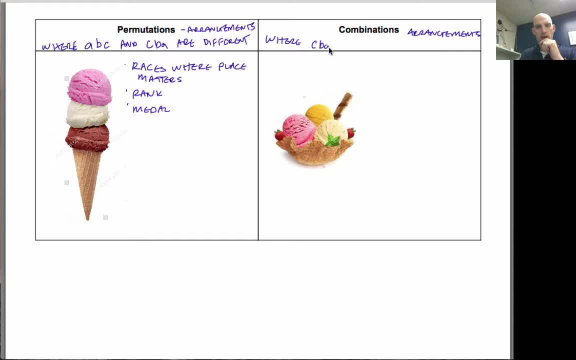 Gold Silver Silver Gold Silver, CBA and ABC are the same. So I put a bowl here because you've got everything inside the bowl and you're not restricted Like I can eat from here or there. They all kind of mix together. 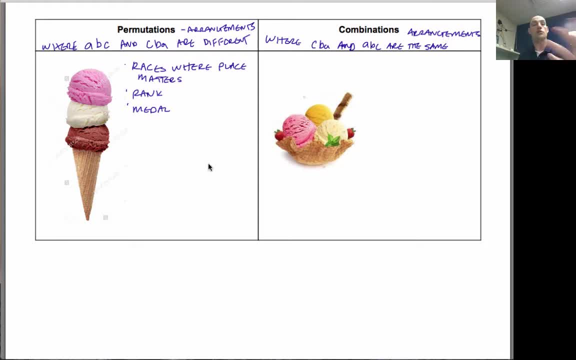 An example of what could possibly be combinations used for Forming groups or committees: Picking top five, no rank. Okay, so picking the top five students in the class but no rank assigned. It's not like first, second, third, fourth, fifth. 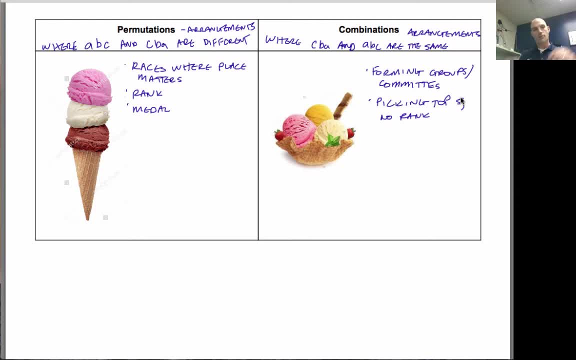 It's just: we need ten, We need five, We need eight Permit two Permit three Permit four Permit five. Here goes. This is when the order is distinct And you're ranking things and there's a specific way they have to be arranged. 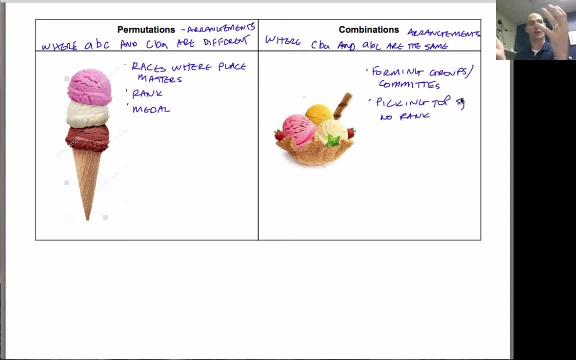 Combinations is more like. we have this group, You're part of the group, You're good. Here's what the formulas look like. For example, it would be n factorial- And if you don't remember what factorials are, three factorial is equal to 3 times 2 times 1.. 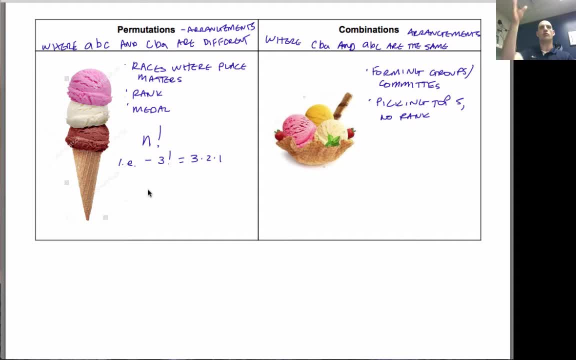 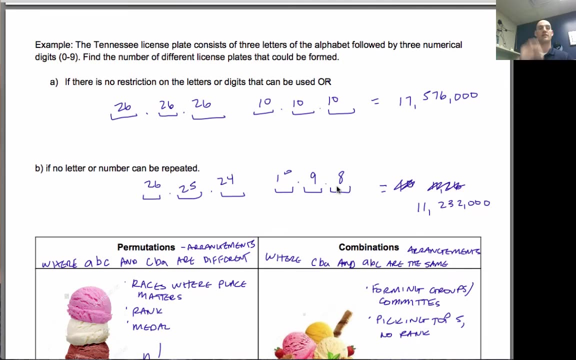 So, whatever n is, you start with n and, in descending order, you multiply every single number or every single number after it. Okay, Uh, so when we're doing our license plate problem, this was a form of a factorial right. So 10 times nine times eight, So 10. 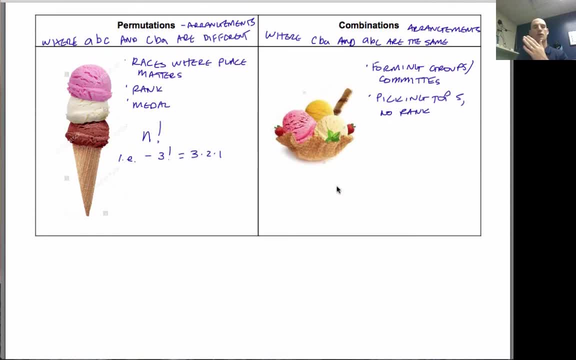 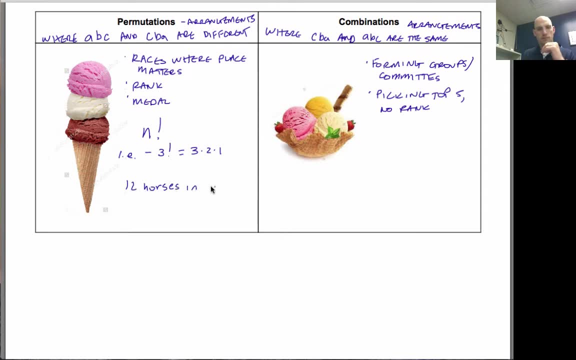 factorial be 10 times nine times eight times seven times six times five times four. Well, think about it like this: 12 horses in a race, How many ways to finish? Well, if you think about that for a second, as they're crossing the finish line, right, Cross the finish line. 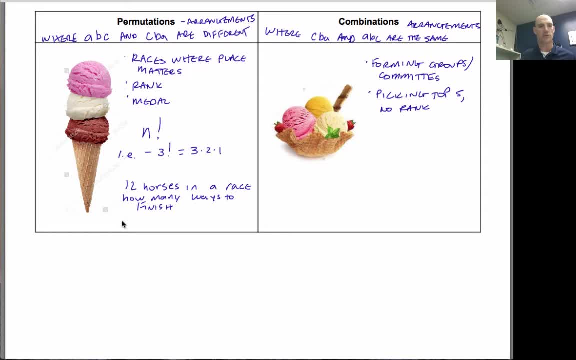 How many horses could come in? 12?. How many horses could come in first? Well, there could be 12. after that first horse finishes, How many options are there for second place? There's 11.. Those two are done. How many options for third? 10 times. 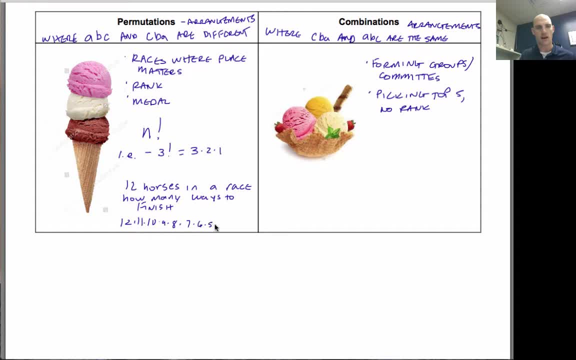 nine times, eight times, seven times, six times, five times, four times, three times, two times one As they finish. there's less options for who could come in that place, because the first place horse doesn't circle back around. It could come in fifth place Also, it would. 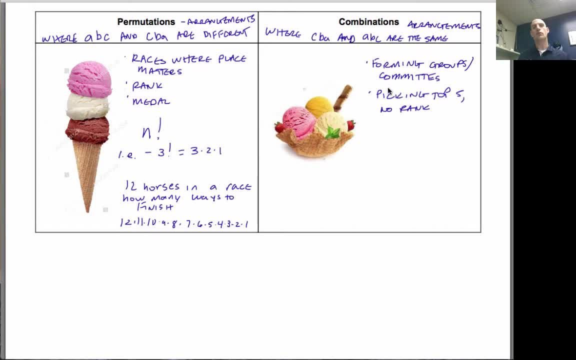 be ridiculous, right? Okay, For combinations, we're going to start the same way. Let's say: you've got five people and you want committees of two. How many different committees of two are there? Okay, That doesn't, it doesn't matter. Like I'm not saying: you're the number one, you're number two. I'm saying: 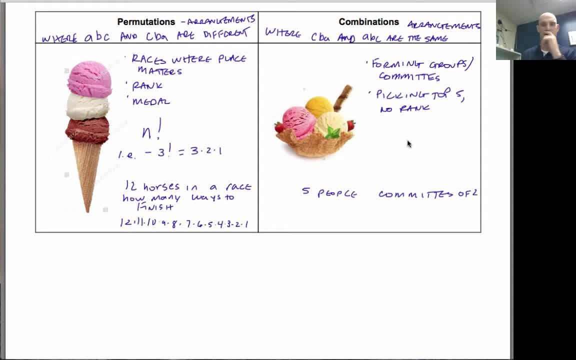 you got two people in a group go with it, Okay, And so what happens is the second horse is going to come in first, So you're going to start with the same. we started with the same formula because, ultimately, let's let's think about the horse example for a second. 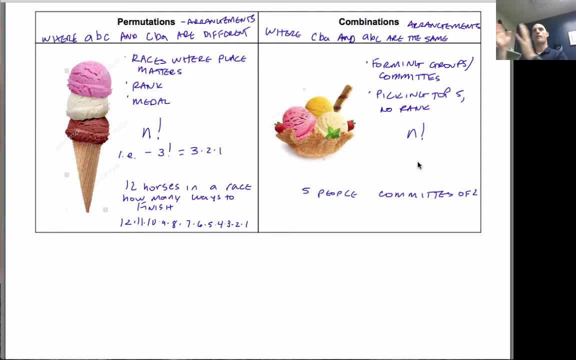 If we're ranking them 12 times, 11 times, 10 times, nine times, eight down the line. But let's say for a second, it didn't matter, This was a qualifying round, You just got to finish in the top five. This is what happens in the first part of the Olympics, right? 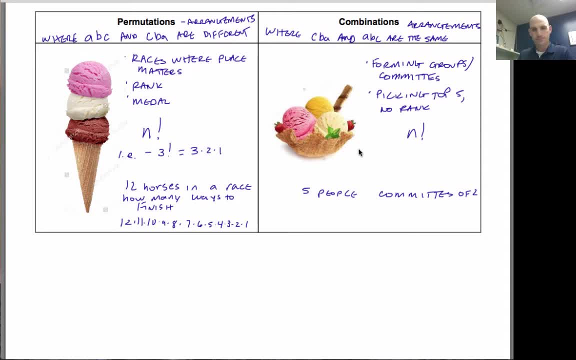 You got to be in the top three of your heat or whatever. For the top three of the heat. what I'm going to do is I'm going to divide by R- R factorial and then N minus R factorial. Here's what it means. This is N objects, So 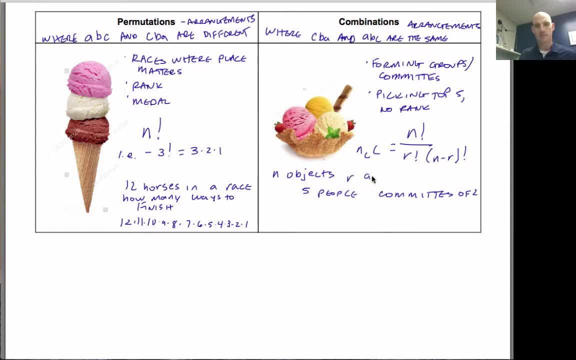 12 horses, uh, and then R at a time. Okay, I pick them all at a time, Meaning I've got 12 horses. pick them five at a time. Well, whether I have ABCDE or BACED, it doesn't. 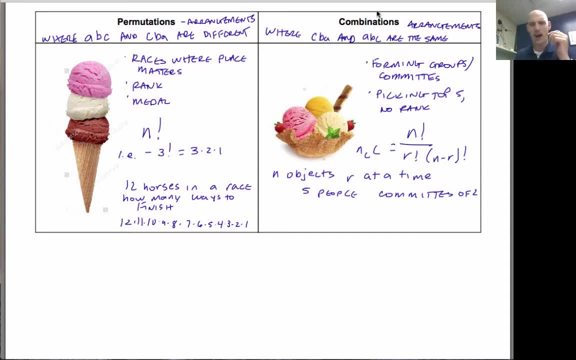 matter, They're all the same right. And so I divide by this part, because this part accounts for the fact that ABC is equal to CBA. So in a combination it's important, because you're saying: I've got all these choices, but ABC and CBA are the same, So I have to eliminate that one. I'm counting. 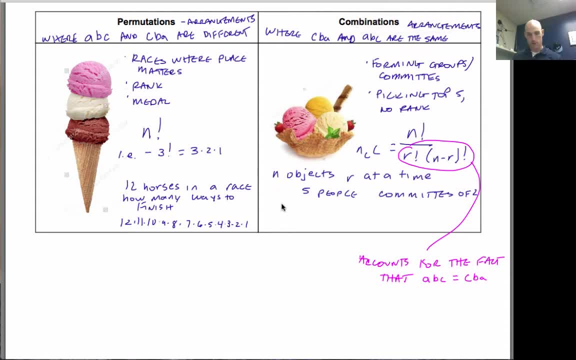 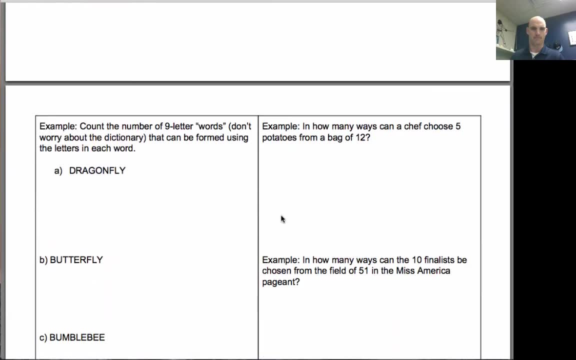 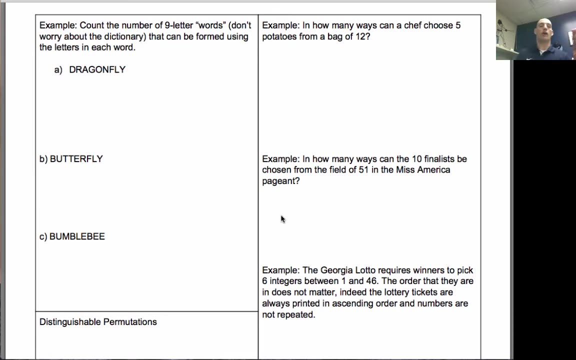 so let's work on some problems that are going to help us determine the distinction- that's sometimes the hardest part- and then apply the formulas to see what we get. start this way some of the common terms- terminology in combinatorics is words. all right, what does? 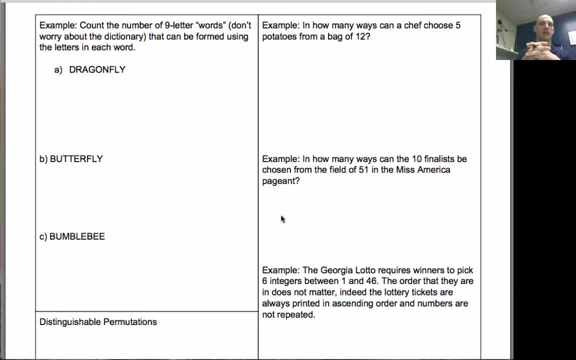 that mean. so by words they're saying arrangements of letters. so it says: count the number of nine letter words. don't worry about the dictionary meaning. it doesn't actually have to be a word. that can be formed using the letters in each word. let's look at the word dragonfly. 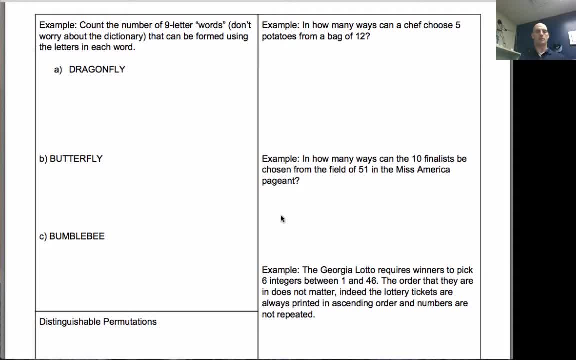 and so for me this comes down to arranging all nine letters. and how many ways can we do that? and so it's nine bins, right? two, three, four, five, six, seven, eight, nine. we'll think about this for a second. it's like scrabble, right you got. 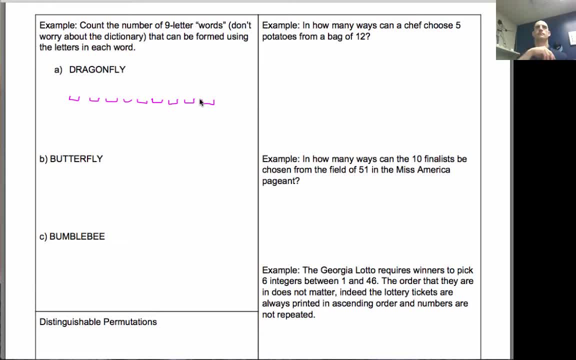 all the. you got all the. you got all the piles in a little bag. you pull one out. how many options did you have, right? so you had nine, then that one's already been used. so then, how many you have when you, when you reach back into the bag? 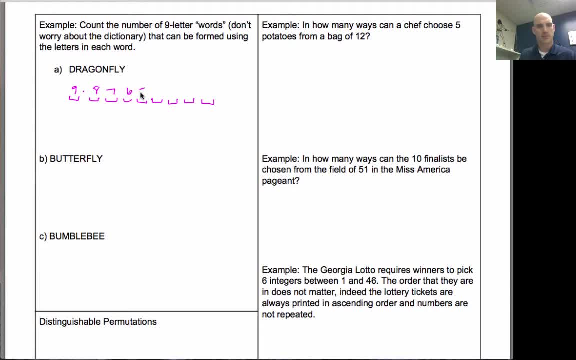 times, eight times, seven times, six times, five times, four times, three times, two times one. the shorthand way to write that is nine. factorial didn't say, it said arrangements of letters. doesn't talk about um committees, doesn't talk about, you know, not being repeated, cause really you know. 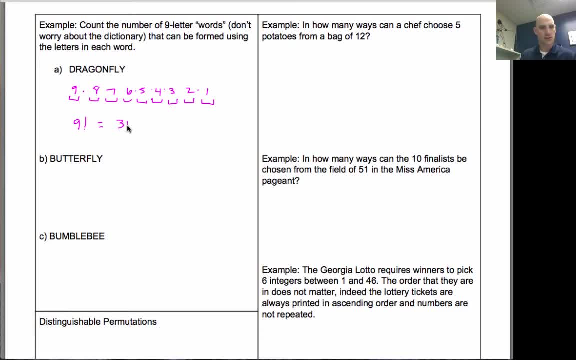 that's. this is straightforward. so 362, 880 ways. so let's look at this next problem here, the word butterfly. so if we look at the word butterfly, what are the considerations that we need to make? think about the bins, right? so one, two, three, four, five, six, seven, eight, nine. so nine bins with also two, three, four, five, and then 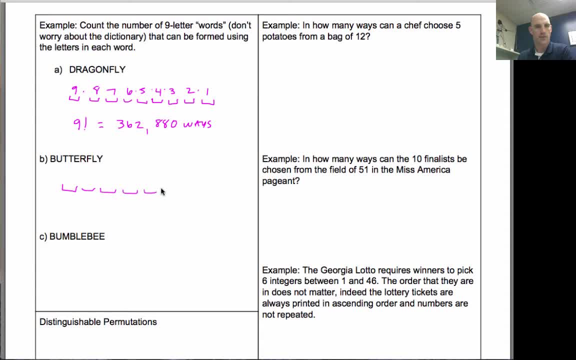 nine bins, also two, three, four, five, and then retire my pie, all your money, into the hard drive and convert it into a comunicated journal, like a journal, which is kind of not what we know about helping readable w. if you six, seven, eight, nine, And when we do this we've got nine times eight times, seven times six times. 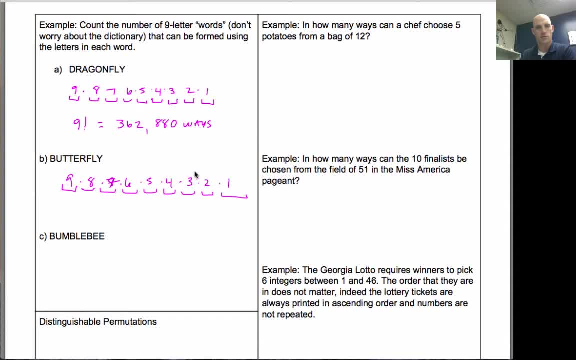 five times four times three times, two times one. But think about this for a second. Let's say we had the word B? U E R F L Y T T and B? U E R F L Y T T. Are those the same or are they? 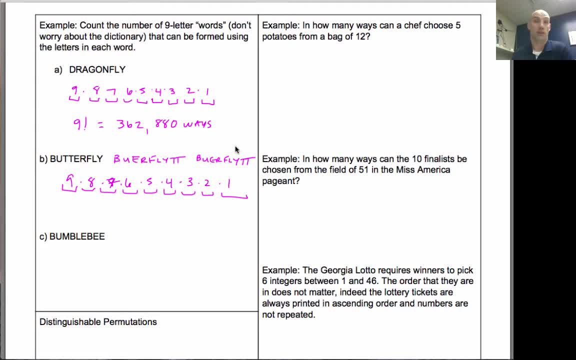 different. You can't tell, can you? Well, what if I told you I switched the T's? What if I told you I didn't switch the T's? How do you know? And so these are what are called indistinguishable objects, And so what we need to do for this one. 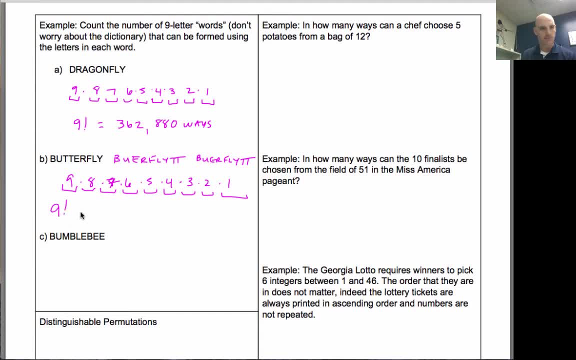 is, we take ourselves our nine factorial and we're going to divide by two factorial, because two factorial is the number of repeated letters, two T's Okay, So let's say we had another like, let's say we had. well, I guess in this next example, 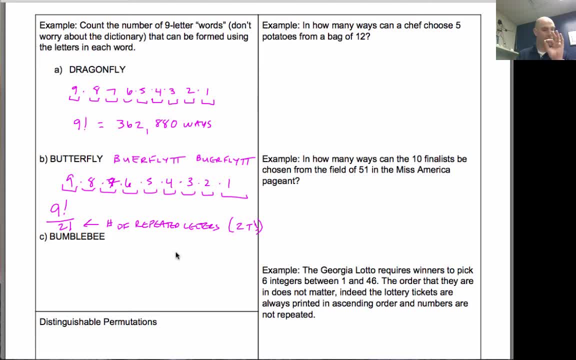 we're going to see that. but we've got this two factorial because it accounts for the fact that there's repeats, And so when I do nine factorial divided by two factorial, it's equal to 181,440.. Okay, So you got to divide by the number of repeated letters. Okay, Let's look at this word. 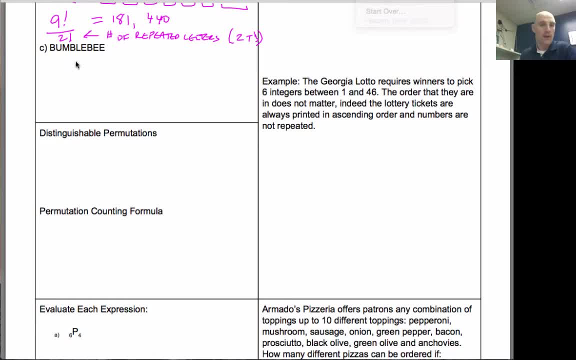 bumblebee In the word bumblebee again, we have nine letters, so nine factorial. And then here are some repeats. I got three B's, And so I've got to divide by three factorial. I also have three E's. 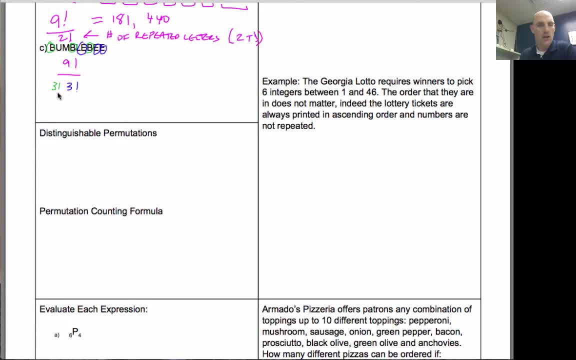 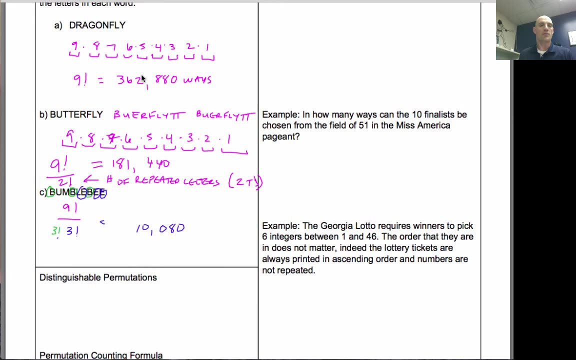 so I have to divide by three factorial. So the numbers on the bottom that we divide by are the number of times a given element is repeated. When I do this I get 10,082.. Take a look at that: With no repeats it's 362,000.. With one repeated letter one time. 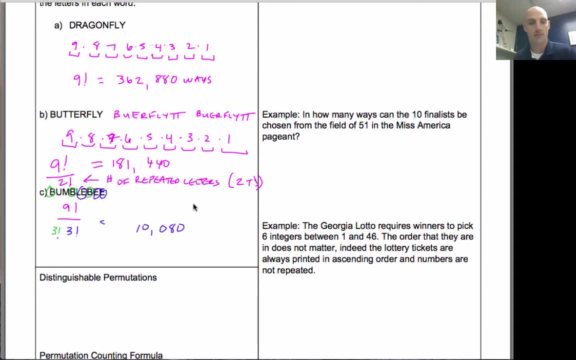 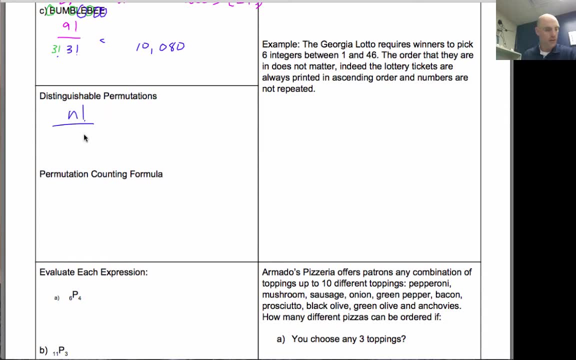 it's 181,440.. When I repeat two letters three times, it's 10,000.. Distinguishable permutations. that's what we're talking about here. And it's N factorial, over N sub one factorial times N sub two factorial. dot, dot, dot, N sub K factorial. Well, what does that mean? 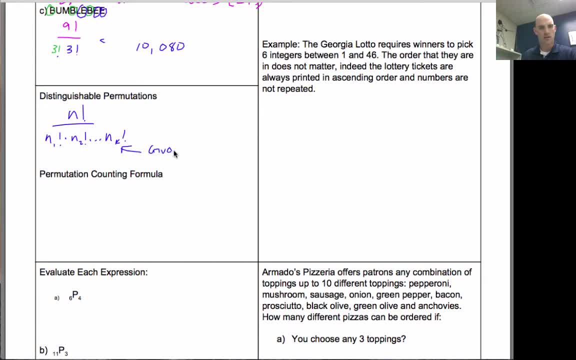 Uh, on the bottom are given- sorry given- objects of a certain kind. Okay, so in that bumblebee example I had two different objects that were repeated three times each Permutation. permutation, uh, counting formula is an object. 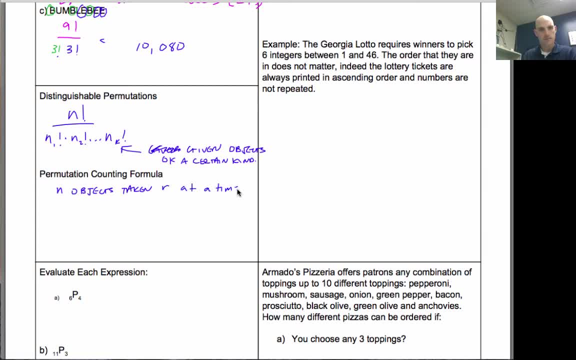 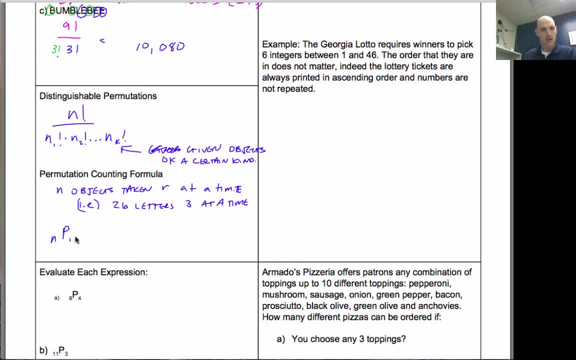 It's gonna take a three at a time. It's denoted NPR or N- factorial over N minus R factorial right. So it would look like this: 26 times 25 times 24.. Well, you're like, well, Mr. 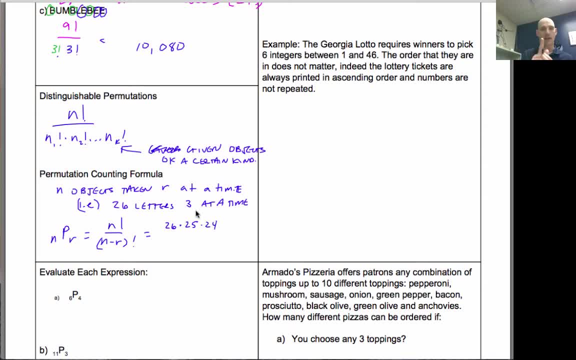 Seris, wouldn't it just be 26 times 25 times 24?? Yes, technically, But really the formula looks like this and it's useful for when we have a larger number of objects or a more complex formula, a more complicated situation. But if we think about it like this, really it's 26 times 25 times 24. 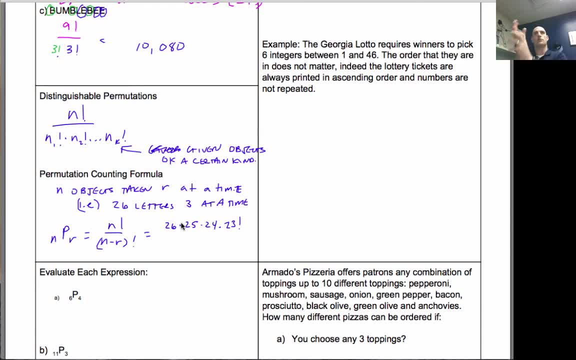 times 23 factorial, because it'd be 23 times 22 times 21,, all the way down. And on the bottom, we're going to divide by n minus r, So that would be 26 minus 3, right, So 23 factorial. 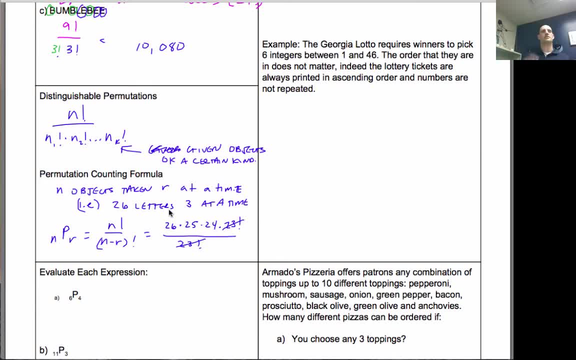 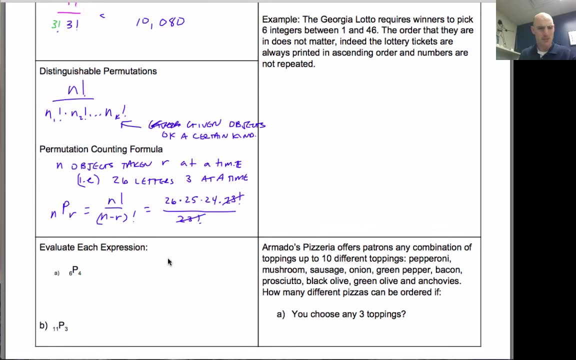 we'll check that out. That's multiplication. it cancels out. So, essentially, what happens is this bin mentality that I was telling you about is I have three objects chosen out of a set of 26, and I don't replace them, So it's 26 times 25,, 24.. So then they asked me to evaluate an expression. 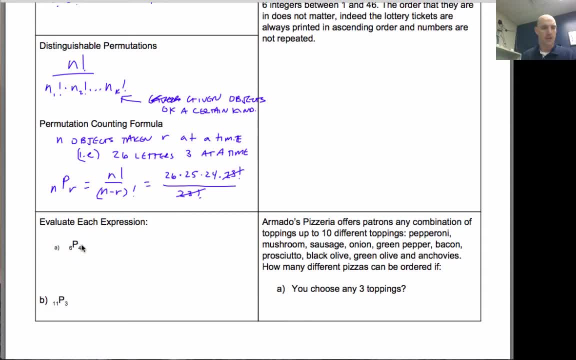 like this: six objects, four at a time. So I'd have 6 over 4 factorial, 6 minus 4 factorial, which is equal to 6 times 5 times 4 factorial. No, 6 times 5 times 4 times 3 times 2 times 1, over and then 6 minus. 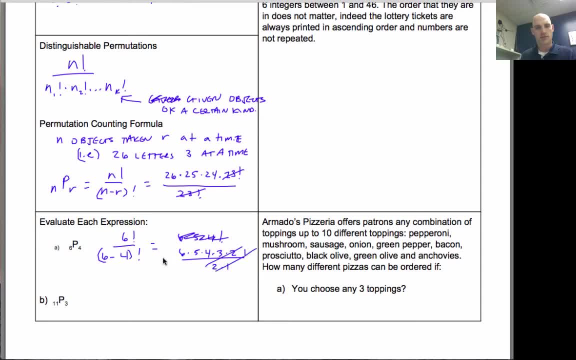 4 would be 2.. So 2 times 1, these cancel out. So I've got 6 times 5 times 4 times 3.. Conceptually, six objects chosen, four at a time, means four bins. the number of choices: six starting. 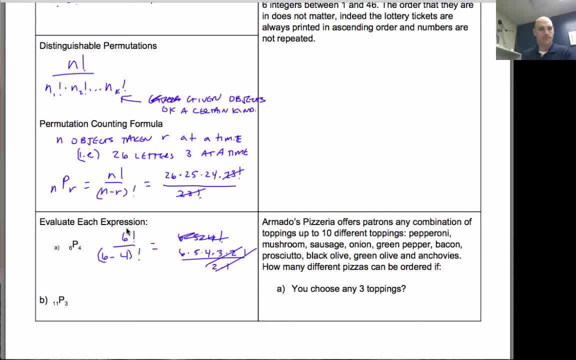 then five because you chose one, four because you chose two, three, 11 objects chosen three at a time: 11 factorial over 11 minus 3 factorial 11 times 10 times 9.. That makes sense. There's three options: times 8 factorial and then 8. 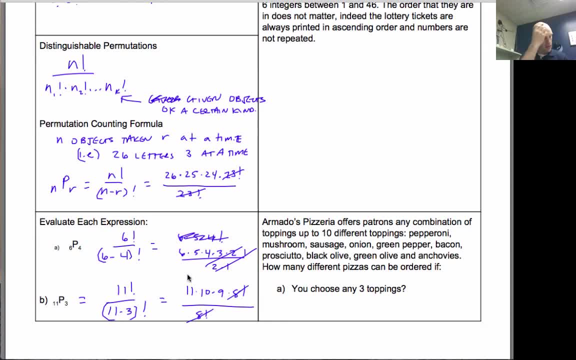 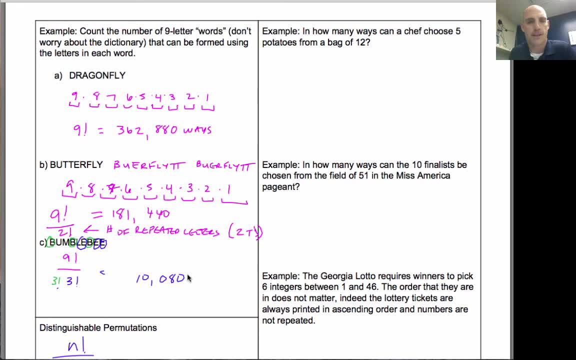 factorial on bottom: gone, gone, done 11 times, 10 times 9.. Okay, so that's the flattened out version. Let's apply this to some situations. How many ways can a chef choose five potatoes from a bag of 12?? So think about it like this: 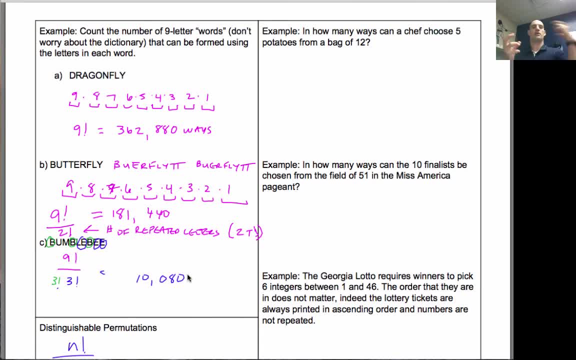 Reach in. You've got potato number one. You've got potato number two. If you're going to put them in a pot, does it matter? Are we ranking them? No, they're not ranked. Not a rank. Okay, we're just choosing a group of five. This is a group, So is this permutation? 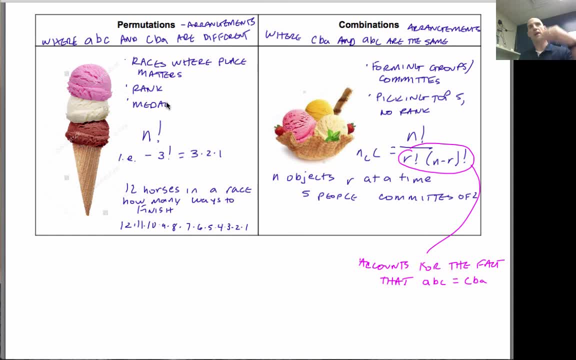 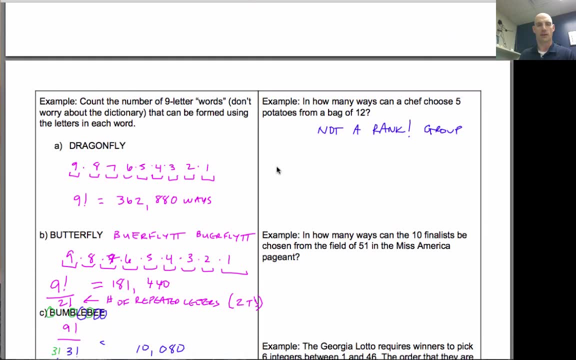 Permutations We'll look up here. Permutations is where we had ranks and medals and races, where place matters, Combinations were committees or groups, And so this: we're going to use our NCR formula And we're going to have 12 potatoes, chosen five at a time. So I'm going. 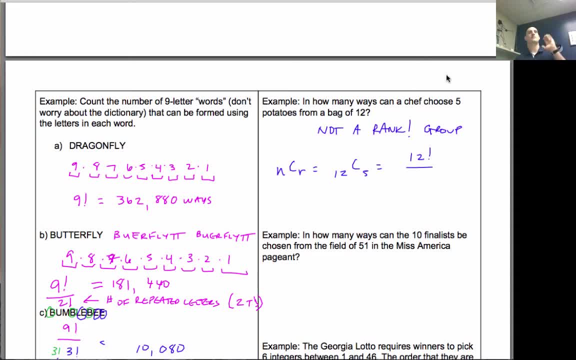 to have 12 factorial, and then I have to eliminate the repeats, because potato A, B, C, D, E is the same as potato D, C, A, B, E. I think I got all the letters right, Okay, And so. 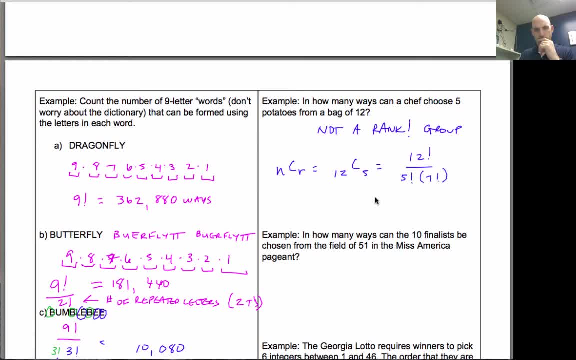 it's going to be over five factorial, And then I have to eliminate the repeats, because we're going to have 12 factorial and then seven factorial. So it's equal to 12, times 11, times 10, times 9, times 8, over five factorial. Okay, And that's the way that I'm. 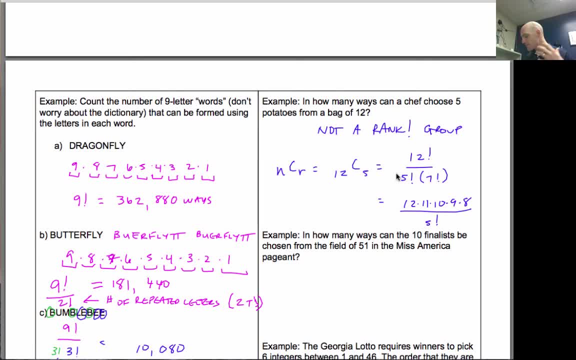 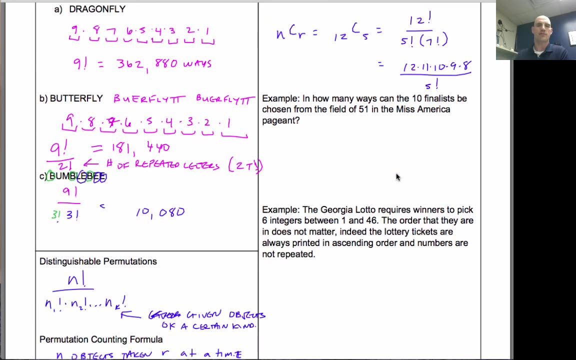 going to do that, But the hardest part of this one is distinguishing exactly what in the world am I going to be using, And so that's a combination formula. how many ways can the 10 finalists be chosen from the field of 51 in the Miss America pageant? 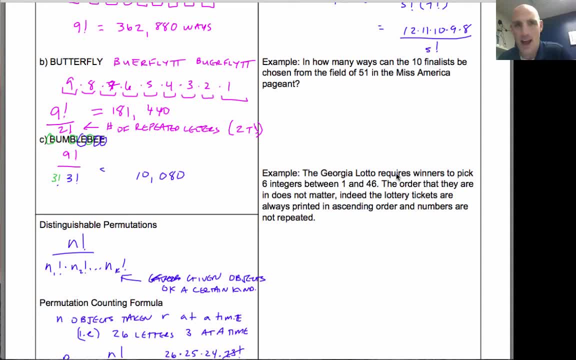 It's asking for finalists, It's not asking how many ways can they finish This one's tricky right. And so I'm really going to have 51 ladies and I'm going to choose them 10 at a time, but it doesn't matter if you've got you know: Alabama, Texas, Missouri. 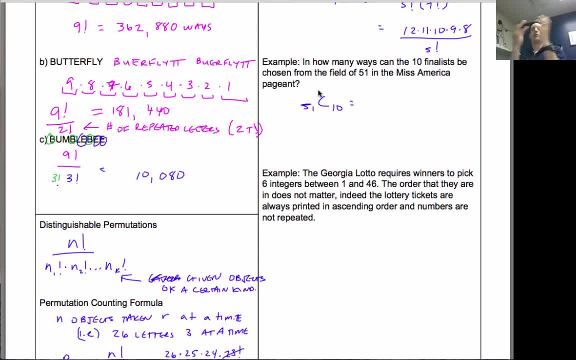 if they're the 10 finalists, you know it doesn't matter what order they came in, or just pick a 10.. 51 factorial over 10 factorial: That's my number of options, And then 41 factorial. that eliminates the rest. 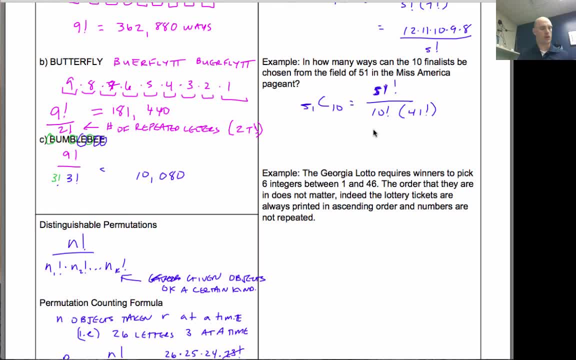 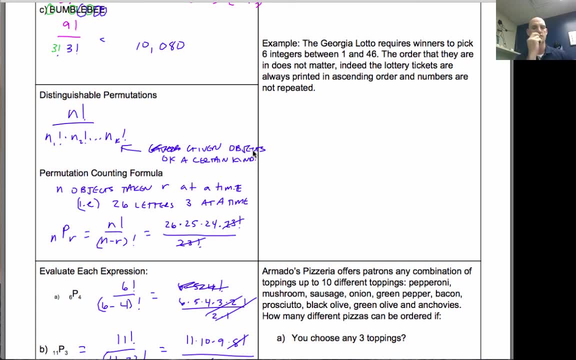 the tail right, So that eliminates everybody who didn't get chosen. Okay, This one's the trickiest of them all so far. The Georgia lotto requires winners to pick six integers between one and 46.. The order that they are in does not matter, Indeed. 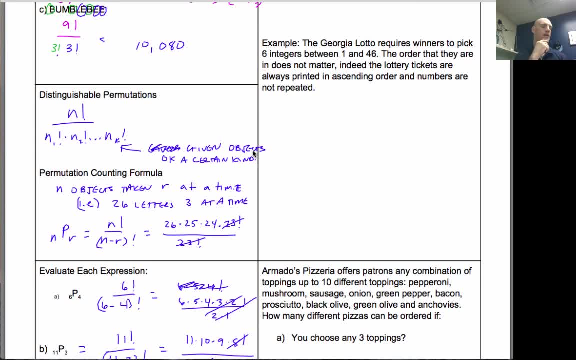 the lottery tickets are always printed in ascending order and the numbers are not repeated. So if I've got one, two, three, four, five, six, guy next to me picks six, five, four, three, two, one, When it prints out they're automatically going to put them in ascending order. So when 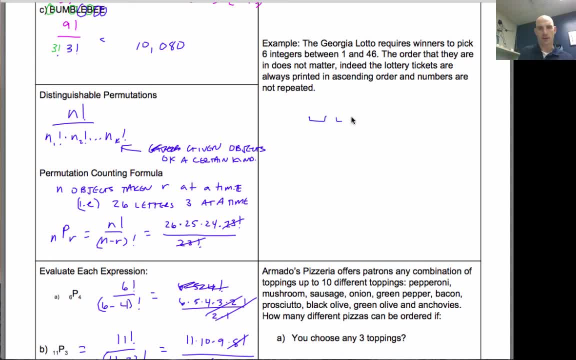 we do this, think about, literally, these lotto balls. They put them in like six different machines, or they might put them in the same machine, depending on how they do this. This one seems to say: they're put, they've got the balls. 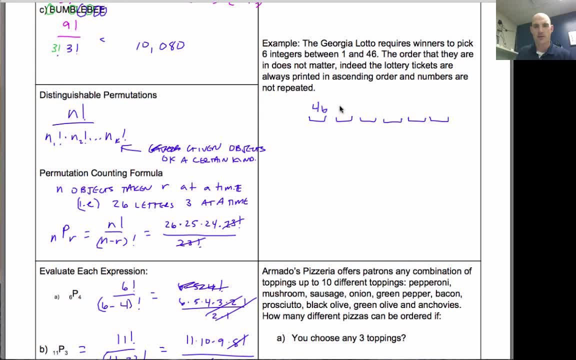 they're in one machine, And so there's 46 options to begin with, then 45,, then 44,, then 43,, then 42,, then 41. But I have to eliminate the repeats, And so I've got to divide by. 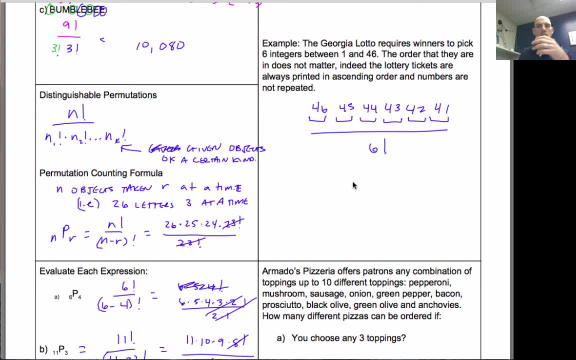 six factorial, because I'm not. I'm saying I've got everything the same. If it's one through six, it's one through six, no matter what order I put them in. And so another way to think of this. so if you're a formulas person, you might say I've got 46, and I'm going to choose six of them. 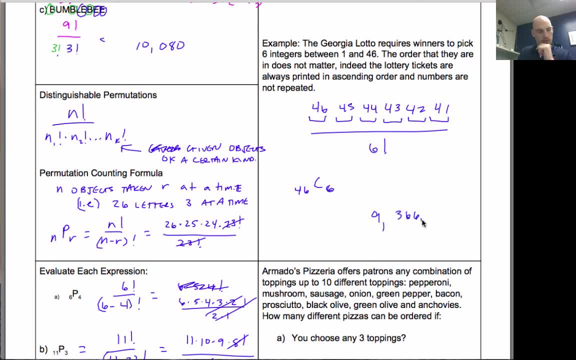 Okay, And that would be 9,366,819.. I've always thought to myself: why wouldn't I just buy every lotto ticket? Well, I got to evaluate: is the winning going to be worth it, right, Okay? 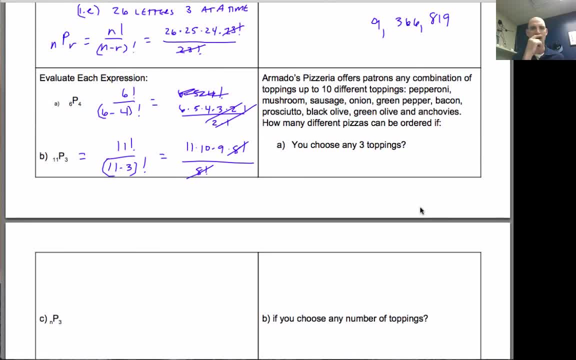 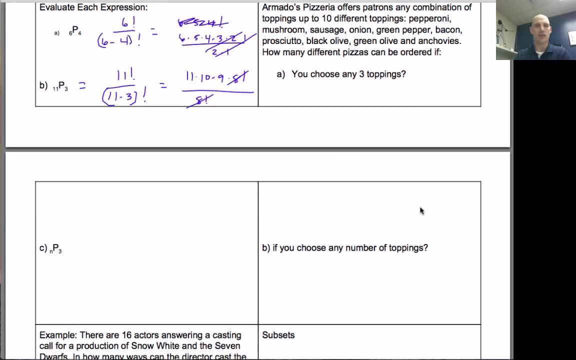 So Armados Pizzeria offers patrons any combination of toppings, up to 10 different toppings: Pepperoni, mushroom, sausage, onion, green pepper, bacon, prosciutto, black olive, green olive and anchovies. How many different pizzas can be ordered if you choose any three? 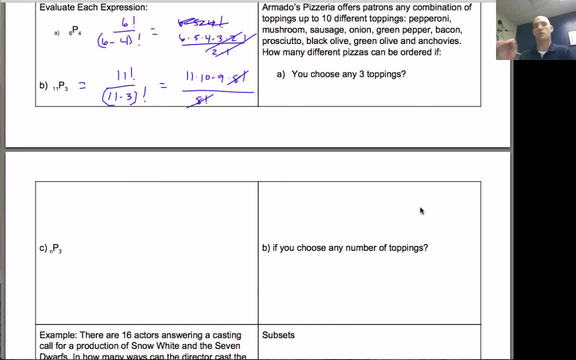 toppings. Once the olives are on there, they're on there. It doesn't matter if you put them on first, second, third, last. That is 10 chopped toppings. choose three And that's going to be equal to 10 factorial over three. 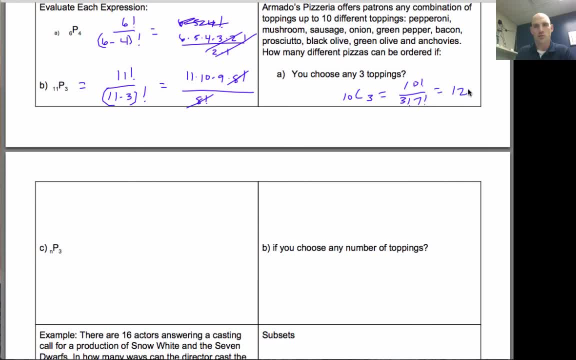 Factorial seven factorial is equal to 120.. There's only 120 pizzas that you can choose, with three toppings. However, if I could put 10 toppings on, think about it like this: I have 10 choices to make: Two, three, four, five, six, seven, eight, nine, ten, right. 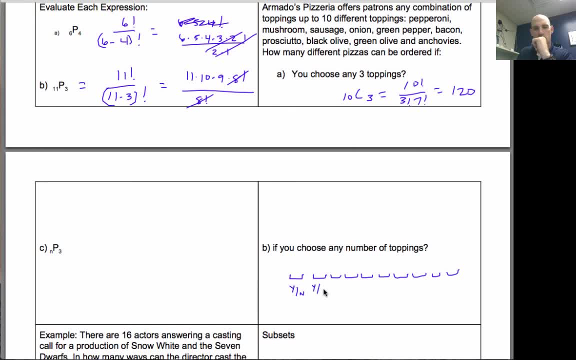 This is a yes or a no, A yes or a no, A yes or a no, et cetera. So in each bin now I'm making 10 choices. You're going down the line and you are telling them what you want on the pizza. But essentially, if you tell: 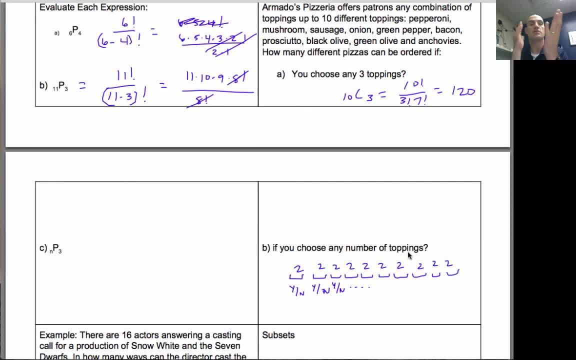 them pepperoni, mushroom and sausage, nothing else. then you said no to seven other things. You really have 10 choices, right? Do I put it on or not? And so I've got two to the 10th power. 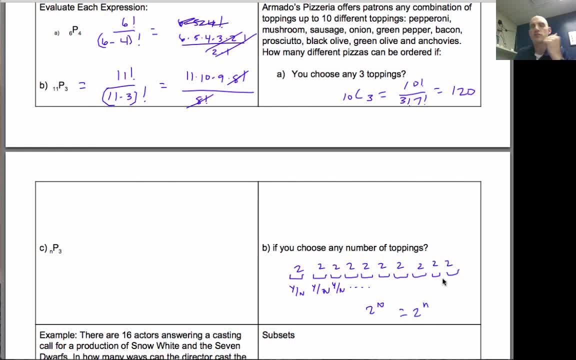 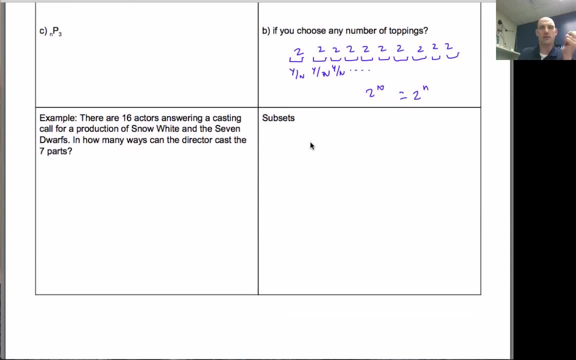 here. right, So it would be two to the N. You could do this with anything, with any number of pizza toppings. right, So that's a two to the N formula. right, So any number of subsets. So a subset would be: you pick six out of the. 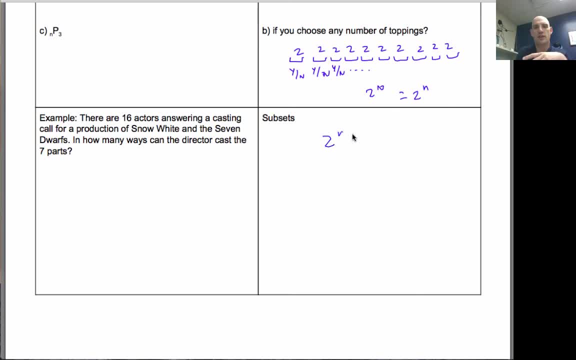 10, and the order doesn't matter. That's going to be a two to the N. N is the number of Or no options. That's the way that I like to think about it. all right, Okay, There's 16 actors answering a casting call for a production of Snow White and the Seven Dwarfs. 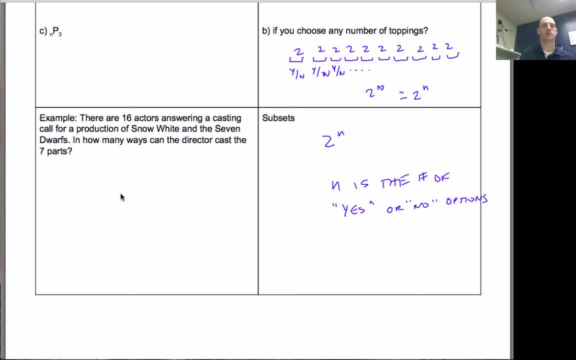 How many ways can the director cast the seven parts? So is it rank, Is it not rank? Well, let's think about it like this: He's casting parts. If I go in for the role of Dopey, and I get the role of Dopey. 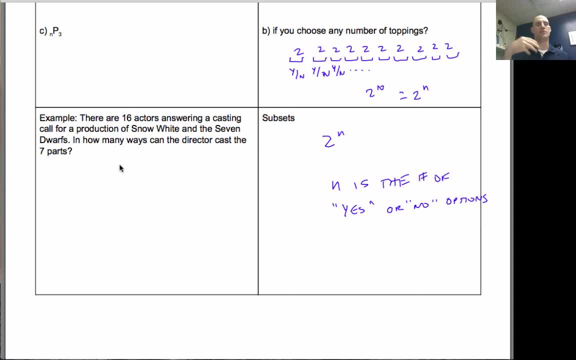 is that different than me getting the role of Grumpy? Yeah, it very much is, And so for this one, order matters, like rank, And so this is 16 people. seven at a time is 16 times 15 times 14..